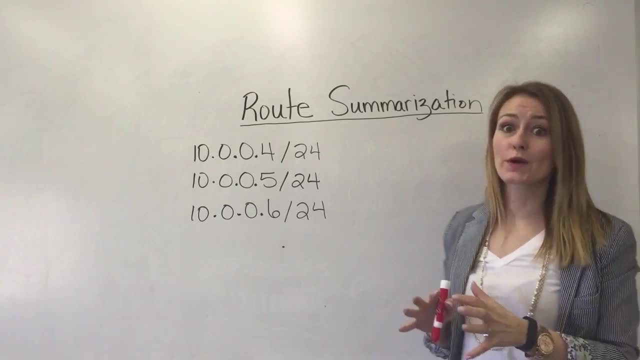 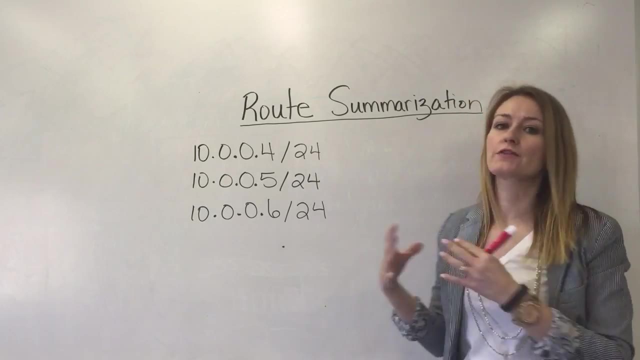 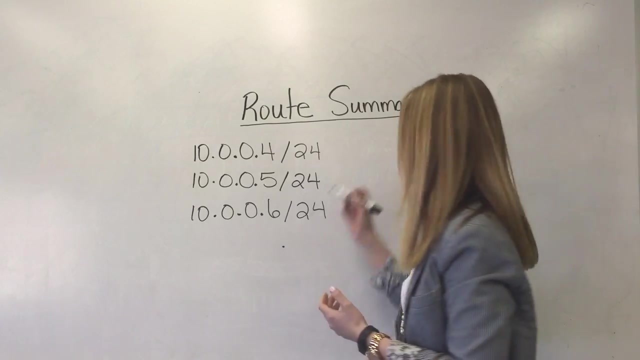 Hi, let's do a quick review of route summarization, also known as route aggregation. Now, the reason why we summarize routes is so that there's less routes in the routing table. So let's say I've got these three IP addresses here that I want to summarize. In order to do the summarization, we have to rewrite the. 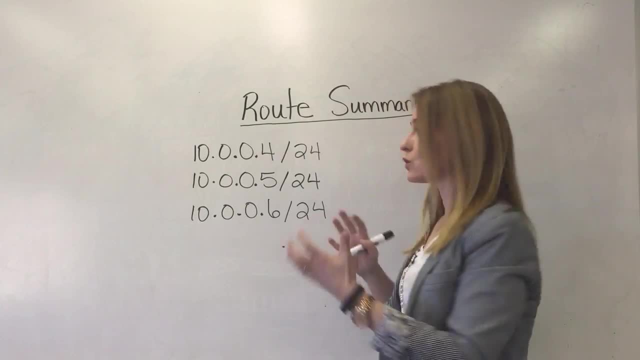 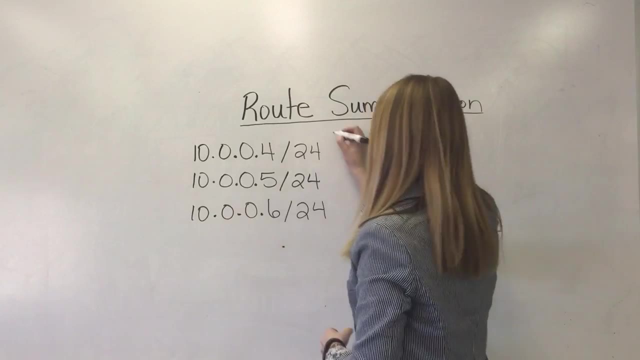 IP addresses out in binary. However, the only aspects we really need to look at is this last octet in this example, because those are the only numbers that are different, So I'm going to take the first three octets and leave them as is. 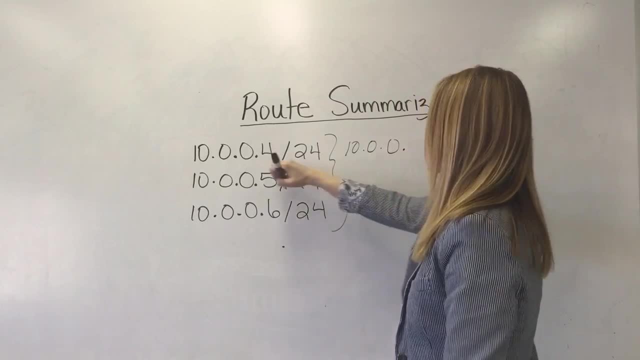 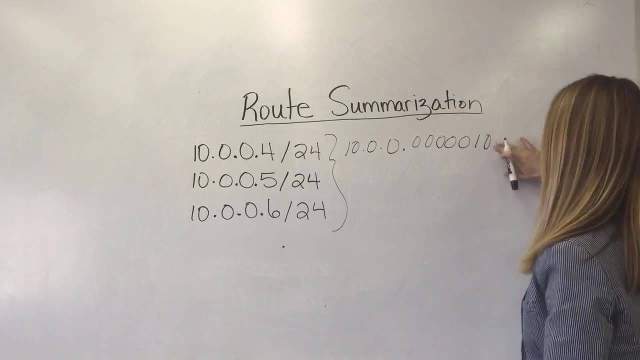 and then I'm just going to convert the last one. So to convert four into binary, we get one, two, three, four, five, six, seven, eight. Oops, sorry, Six, seven, eight, That's four. So then five in binary. 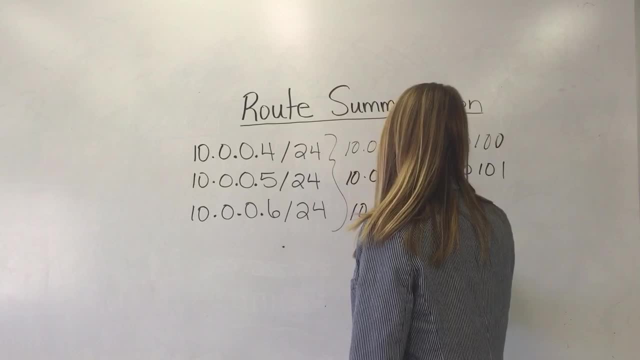 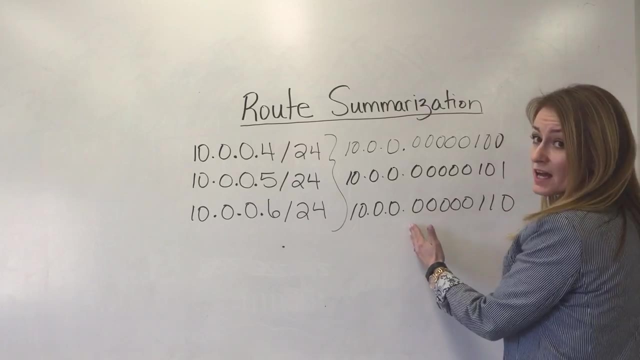 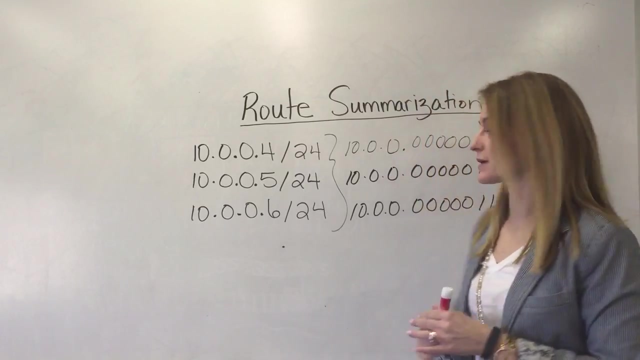 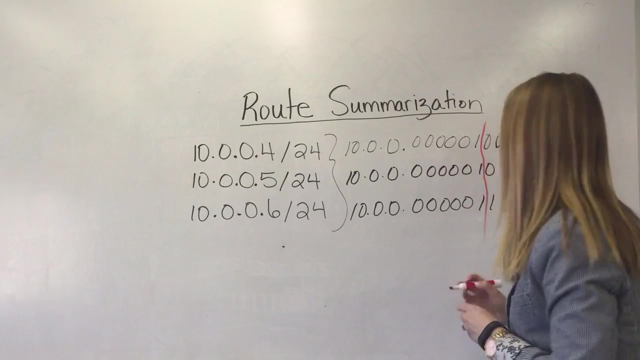 There's five And there's six, So we're gonna analyze this last octet Now. the only thing we care about is where these IP addresses become different. So all the way up to here, they're identical to one another. So let's draw a line where they become. 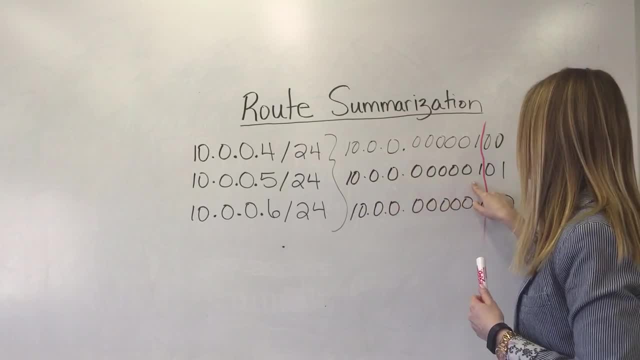 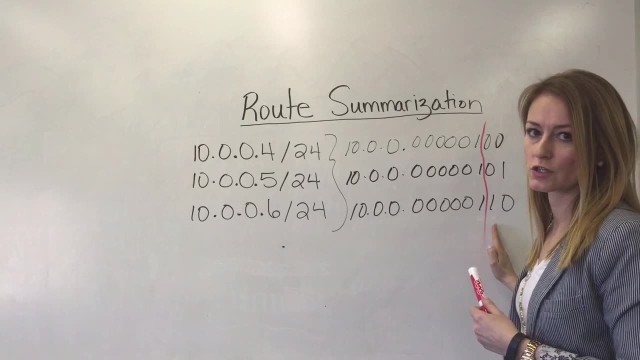 different. Notice: the first three octets are identical. Now in the last octet they're all prefixed with a bunch of zeros, And the first octet is a one, and then, at this point, is where they change. So we just need to rewrite our IP address, taking everything from the line to the. 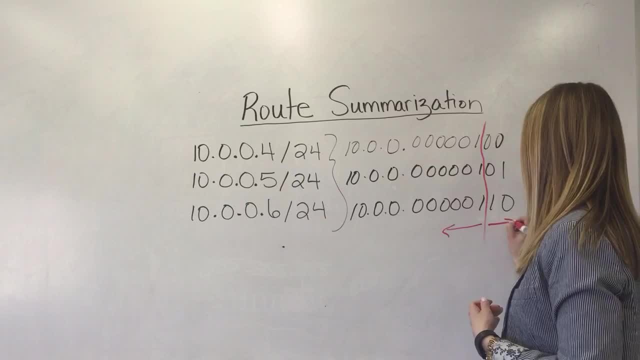 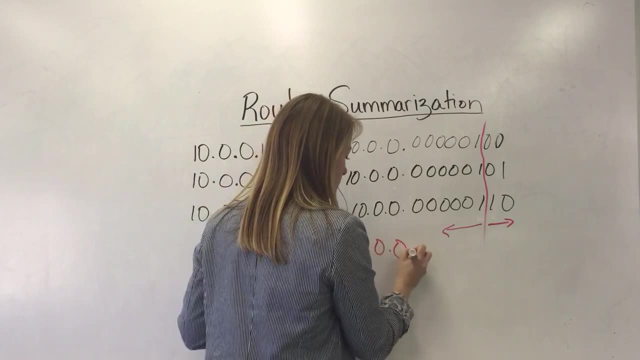 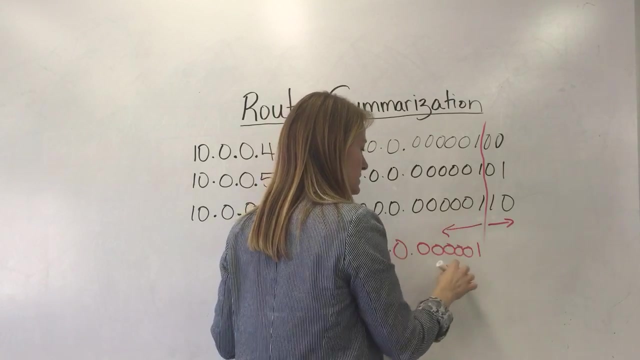 left and keeping it exactly the same, and everything from this line to the right, they're going to become zeros. So we end up with 10.0.0 and I'm going to keep this in binary for now. So that's this right. it stays the same. and then 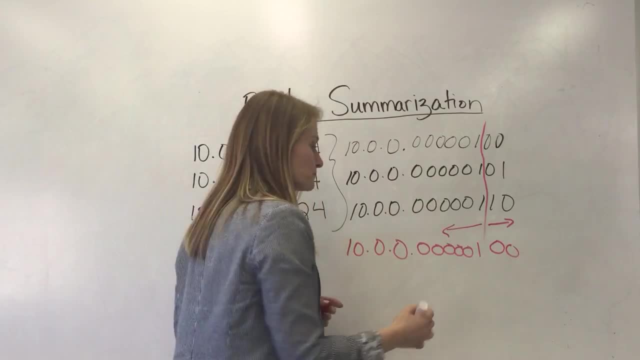 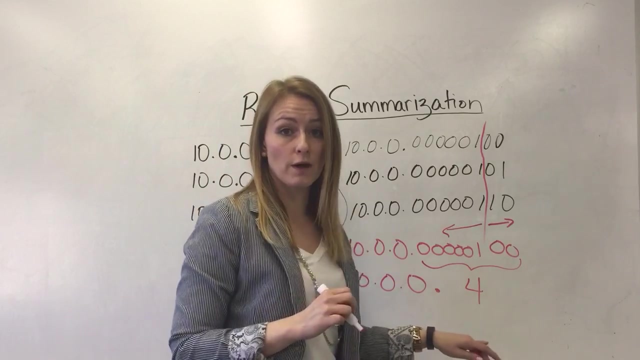 everything to the right of the line just become zeros. So we, when we convert that into decimal, this becomes 4.. So our IP address of our summary route is 10.0.0.4.. Now we also need to determine the subnet mask, So everywhere in the IP address.